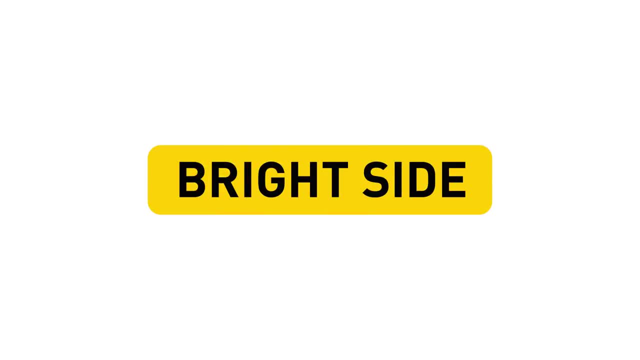 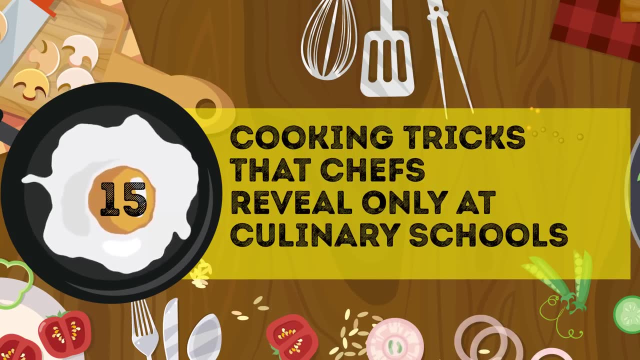 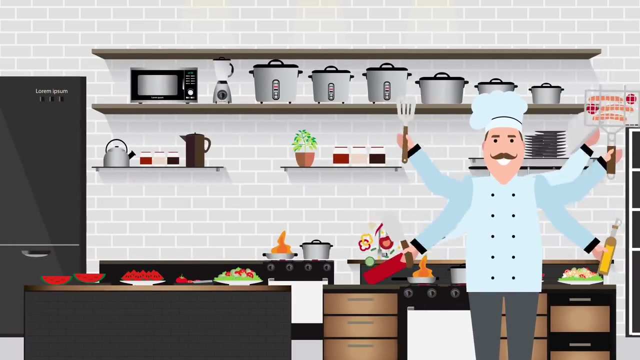 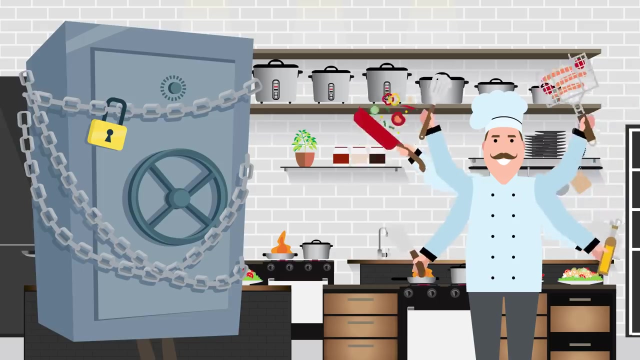 15 Cooking Tricks That Chefs Reveal Only At Culinary Schools. How do restaurant chefs manage to cook delicious culinary masterpieces so fast? Professional chefs usually keep all their cooking tricks a secret and share them only with their students. However, we have managed to find out some drops of cooking wisdom. 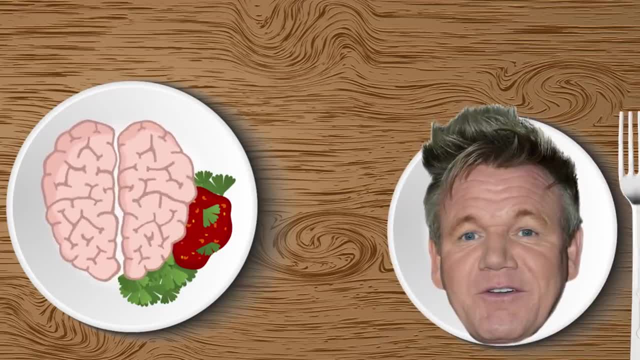 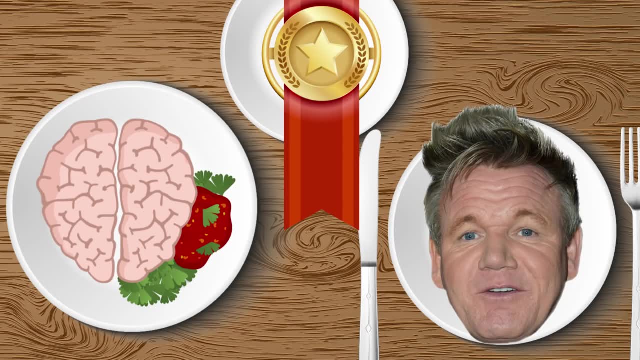 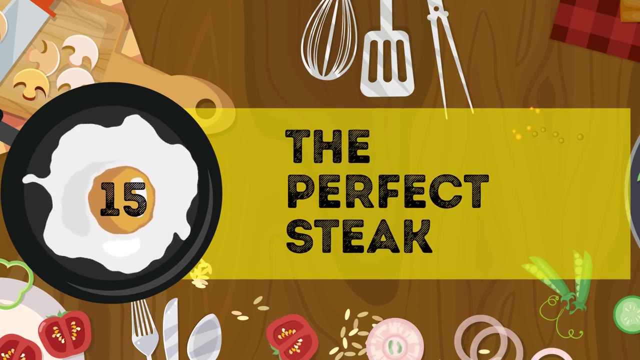 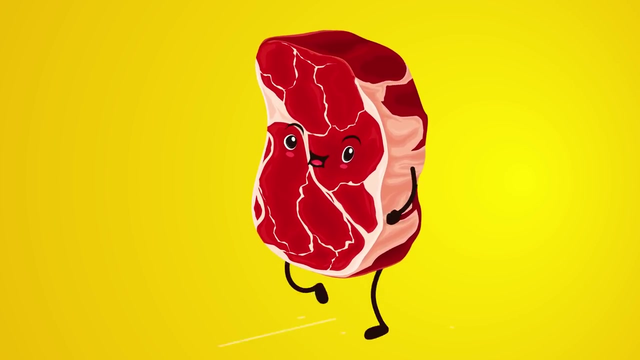 These secrets will help to make your dishes taste just as great as Gordon Ramsay's, or even better. Also, you will be rewarded with the most unusual cooking trick you have ever heard of 15.. The Perfect Steak. Starving you, hurry home thinking of that perfect piece of meat that will make such a wonderful steak. 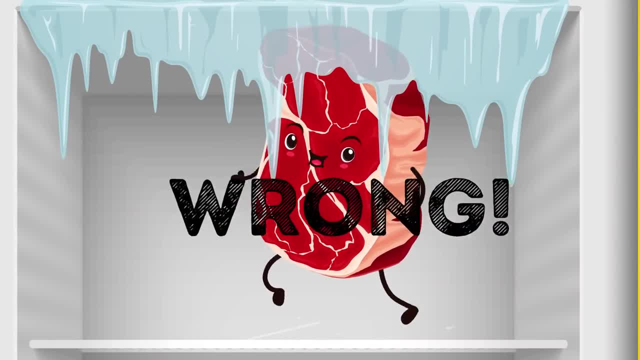 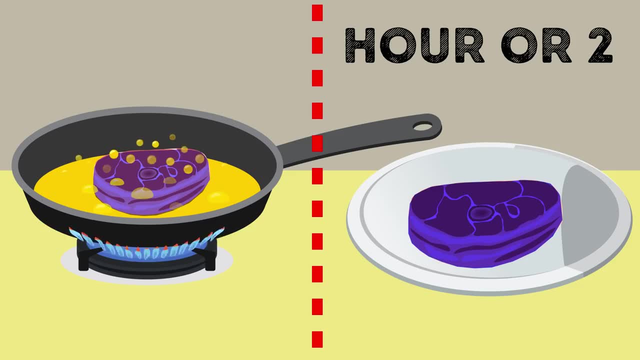 It's still in the freezer, but it shouldn't matter, right Wrong? Don't fry a piece of meat that you've just taken out of the fridge. Leave it for an hour or two before cooking to let it come up to room temperature. 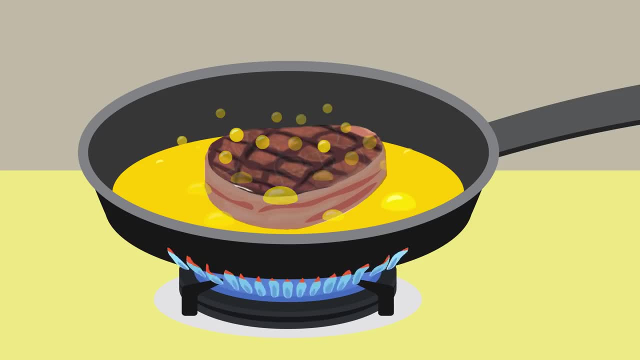 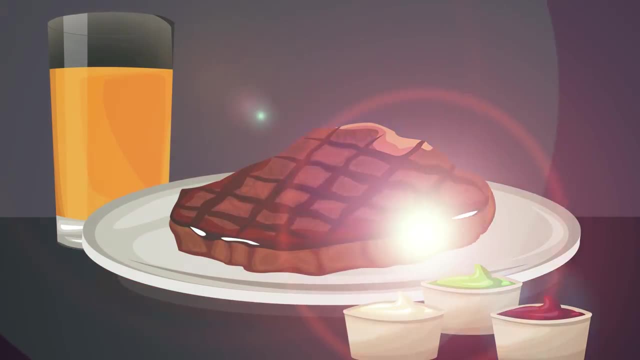 Now you'll fry the meat evenly and get a great meal, regardless of how you like your steak done. If you want a beautiful brown crust on your steak, get rid of all the moisture in the meat before frying. So if you're too hungry to wait, maybe it's better to order some pizza. 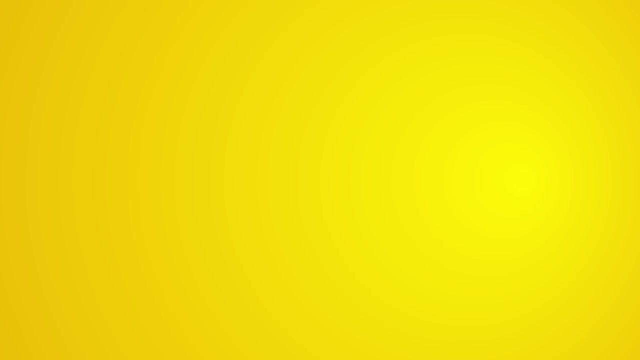 14. The Juiciest Meat. It takes time to fry chicken or pork properly and you can dry them out very easily. To avoid this, many European chefs use a simple trick: They put the meat in a brine. It's very easy to make a good brine. 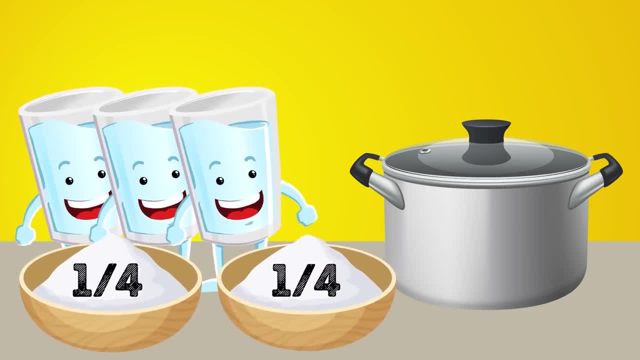 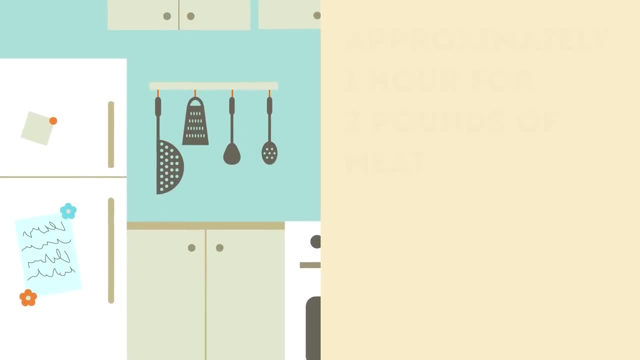 Take three cups of water, add a quarter cup of salt and a quarter cup of sugar, Pour the brine onto your meat so that the liquid covers it and put the bowl in a fridge. The time of brining depends on the thickness of the chopstick. 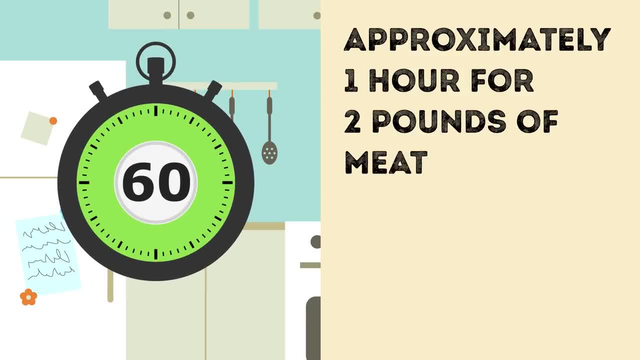 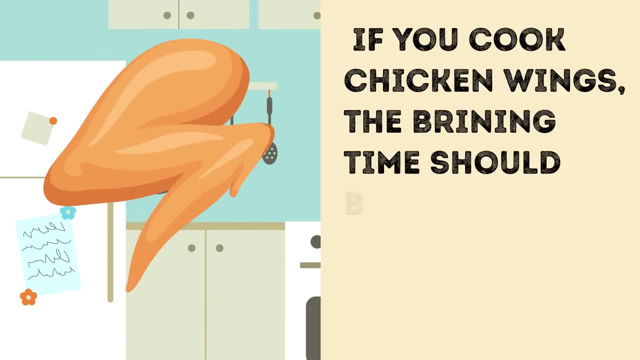 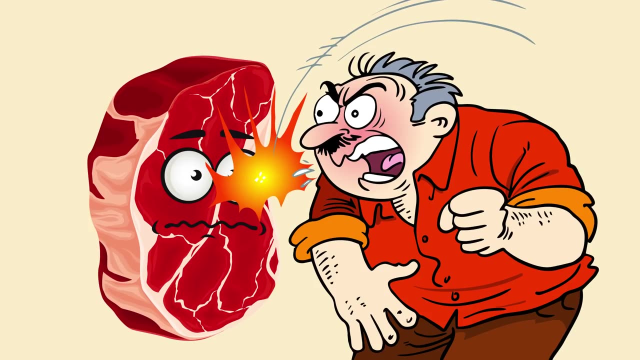 You have approximately one hour for two pounds of meat. Don't leave it for more than eight hours or less than a half an hour. If you cook chicken wings, the brining time should be based on an average weight of one wing. Don't forget to pat the chops dry before cooking. You want them fried, not stewed. after all. 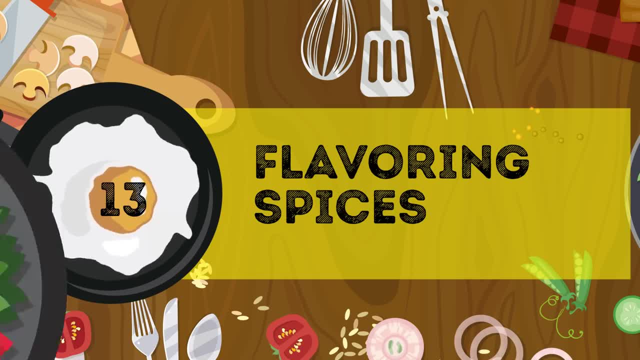 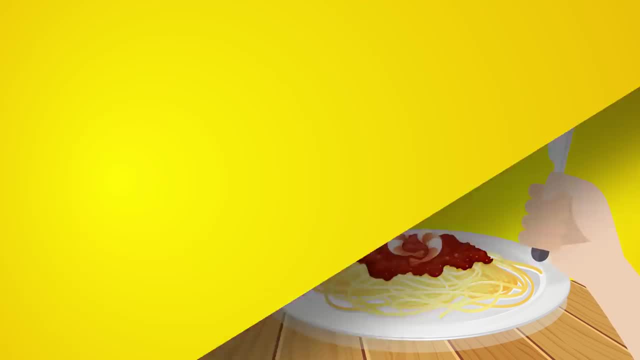 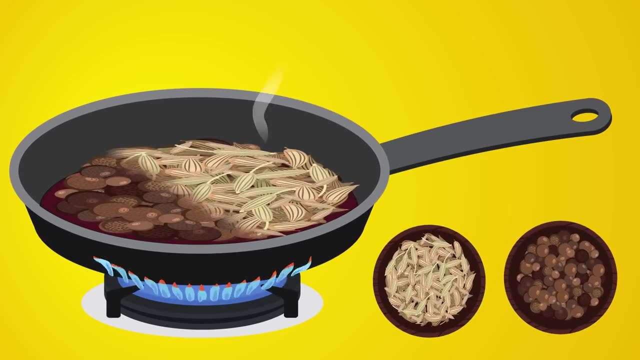 13. Flavoring Spices. If you are that person who likes their dishes savory and full-flavored, this tip will take you to cloud nine. To extract natural flavors and enhance the taste of the black pepper or cumin in your dish, toss them in a pan over medium heat. 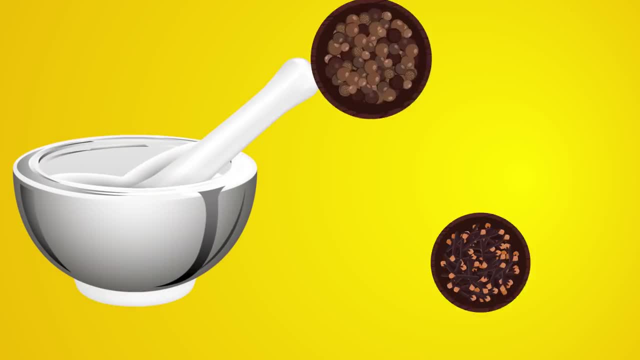 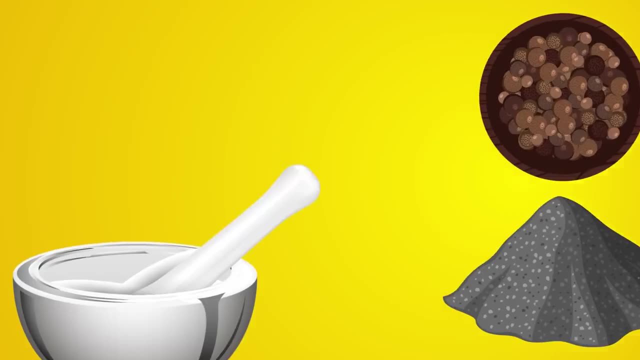 toasting them until they're fragrant. After that, you can use a mortar and pestle to grind your spices. You can substitute ground black pepper with black peppercorns and crack the seeds When you add it to your dish. you'll get a much better aroma and flavor. 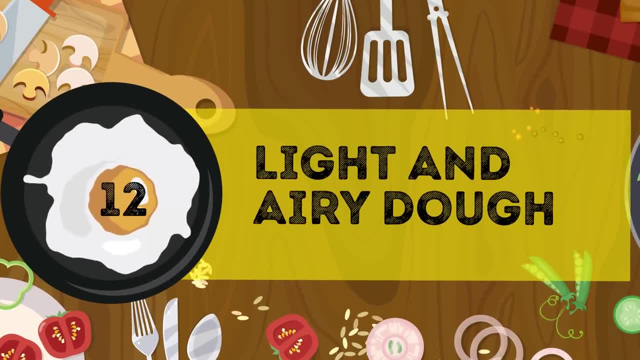 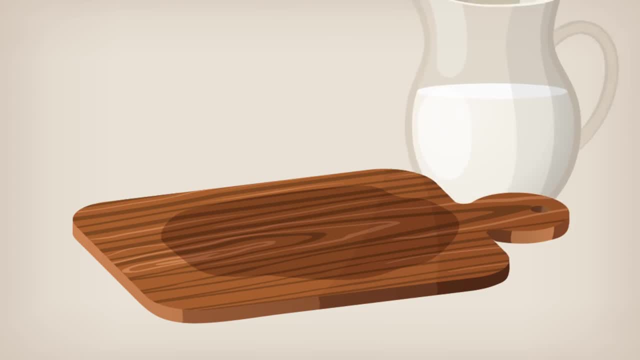 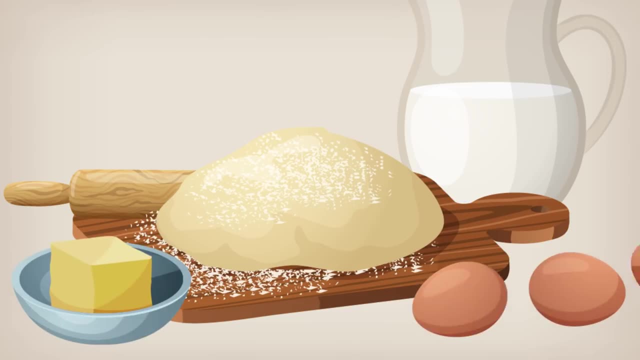 12. Light and Airy Dough- Number 12. Light and Airy Dough. Do you prefer to cook from scratch? Then you prepare the dough yourself. If you want to make it perfect, here is a simple rule: Take the butter and eggs out of the fridge the night before to let them come up to room temperature. 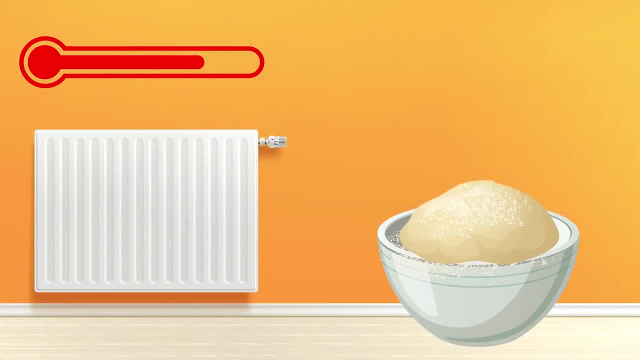 You'll thank us later. What is more, if you use yeast, put the dough in a warm place and wait until it becomes very puffy. The puffier the dough, the better. The puffier the dough, the better. The puffier the dough, the better. 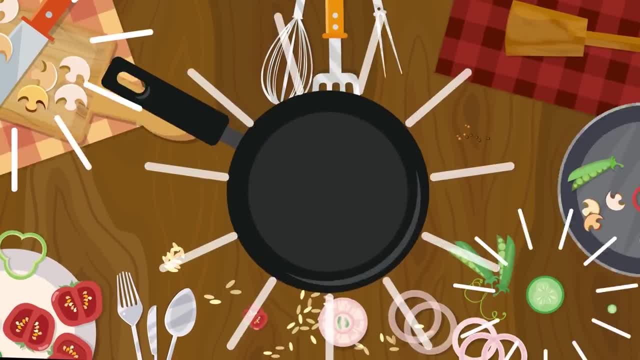 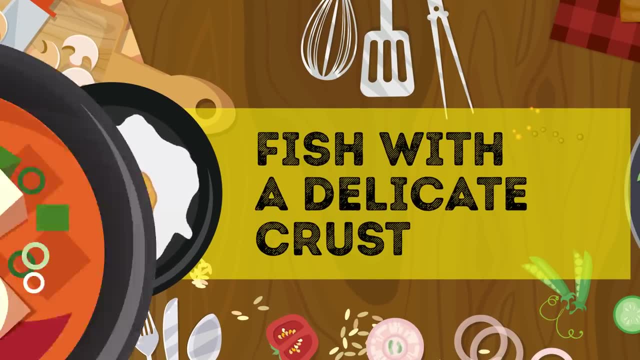 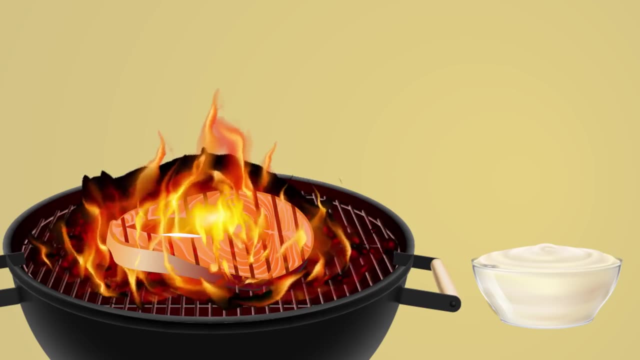 And the lighter the dough, the airier, the pastry. Number 11. Fish with a delicate crust. If you want to fry fish on a grill, Spread some mayonnaise on it to get a tasty, delicate crust. Take a pastry brush, dip the tip in the sauce. 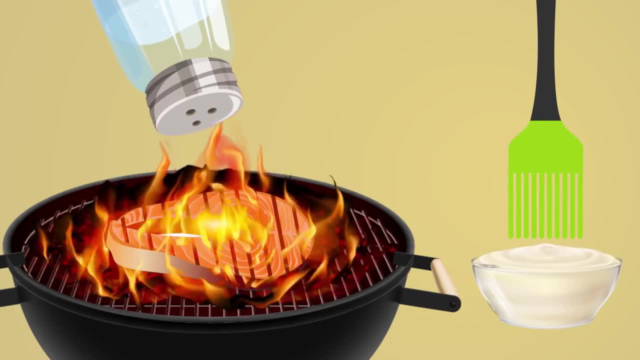 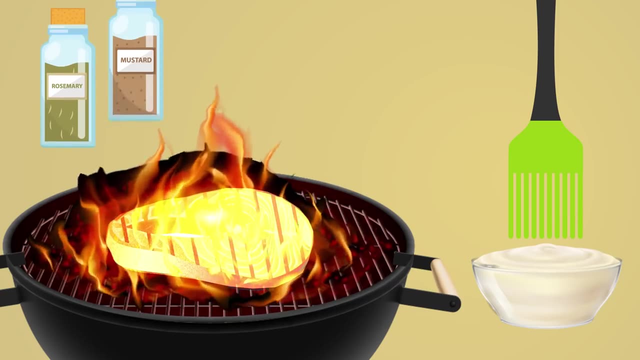 and lightly apply mayo to the fish, Add some salt and then grill it. We guarantee you'll get a perfect golden crust. Use the minimum amount of sauce amount of spices on your fish. It's better to use salt When the fish is done spritz. 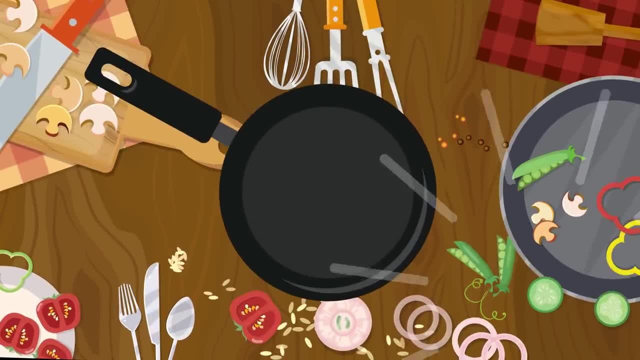 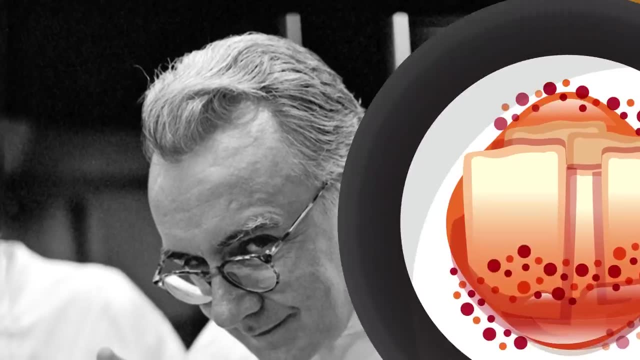 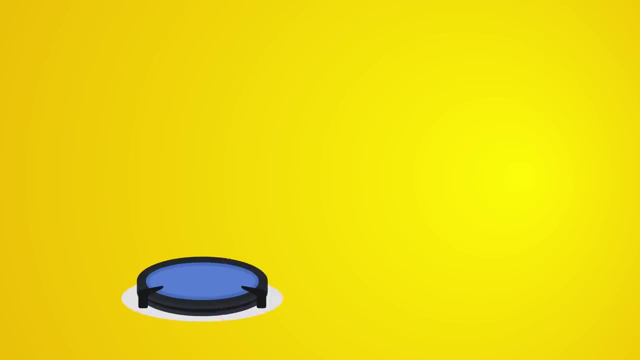 it with lemon juice for the best result. Number 10. Cooking Steak Without Oil. Alain Ducasse, one of the most famous chefs in the world, revealed his secret for cooking a great steak. The steak is placed on its edge because it renders the fat. Now you're able to cook the steak in beef fat Plus. 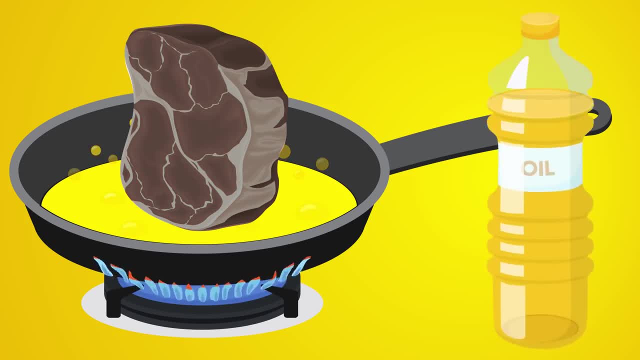 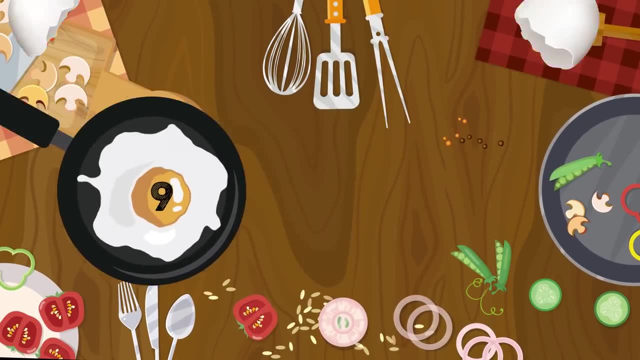 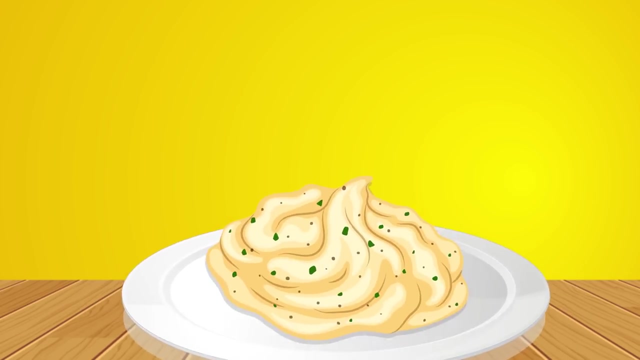 it creates a delicious crust on the edges. Thus, you don't need to use oil while cooking. It's as simple as that. Number 9. Creamy Mashed Potatoes. Mashed potatoes are considered to be ideal comfort food, but let us be honest: When was the last time your potatoes were fluffy and 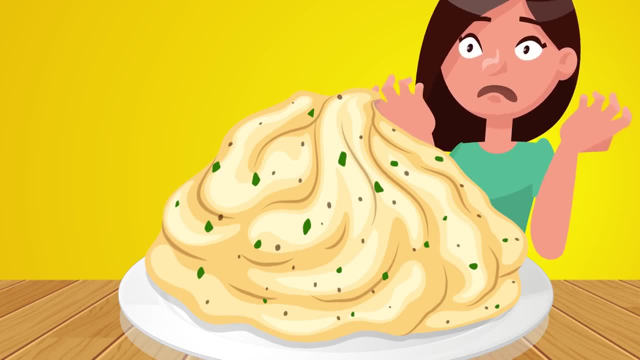 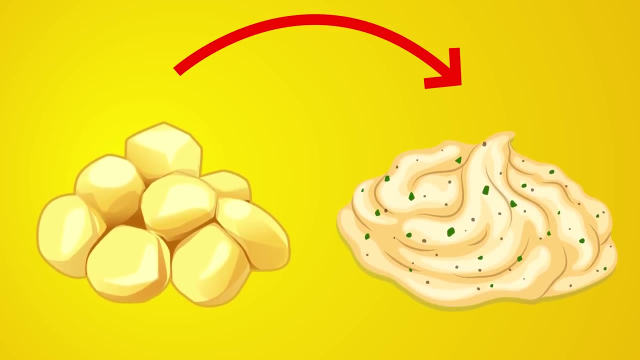 creamy enough. To prepare them properly isn't as easy as it seems, But we have a secret to share. Before turning boiled potatoes into the mashed ones, you need to dry them properly. Just place them in a clean, heated frying pan and keep them there until the remains. 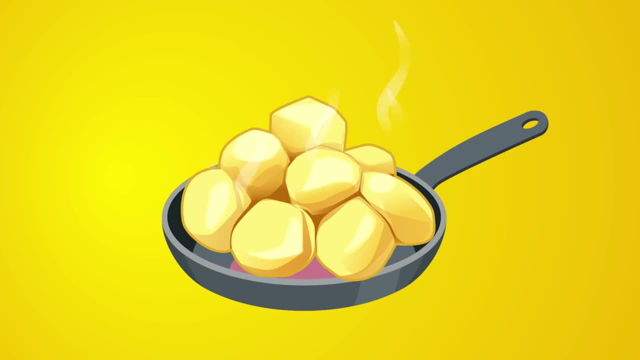 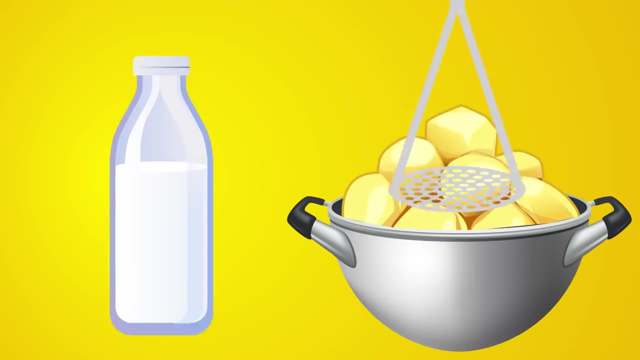 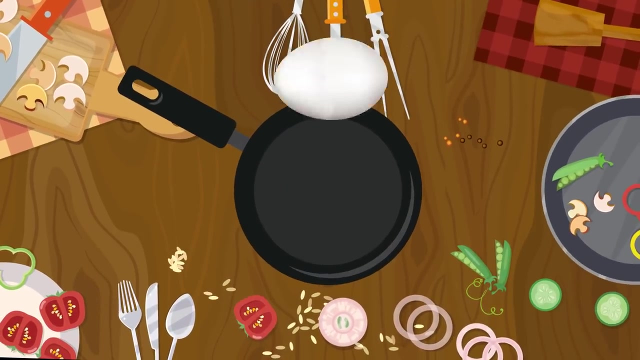 of water dry out. Don't let the heat fry them. When the potatoes are dry, you'll get the best creamy mashed potatoes. A little extra tip To avoid hot milk splashing when you make mashed potatoes, smash some of them in a pan and then add the milk. 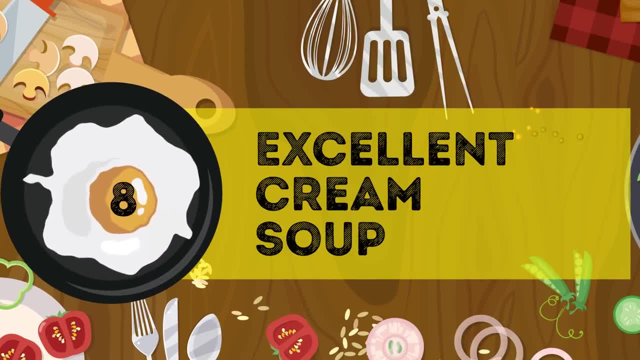 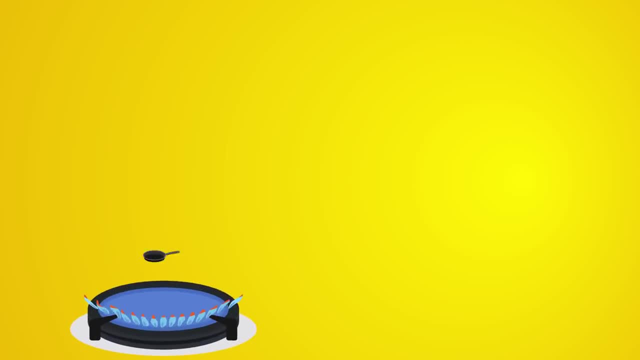 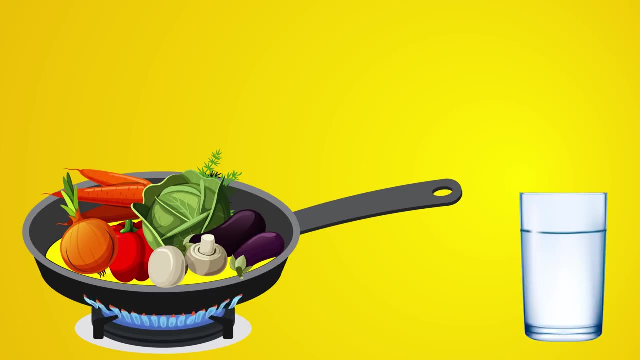 This recommendation will come in handy for the lovers of vegetable cream soup. Right before you start cooking it, fry all the vegetables separately with olive oil, Then add some water or broth. Frying will caramelize the sugar in the vegetables and enhance their flavor. 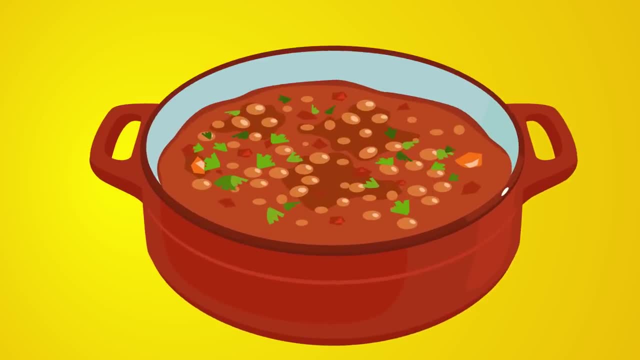 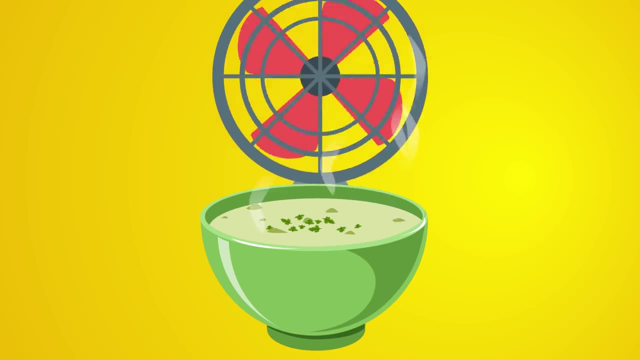 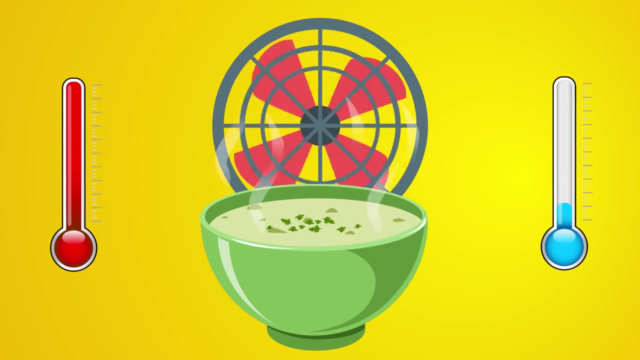 The dish will be exquisite and tasty. The same trick can be applied to a vegetable stew. Please remember one more thing: As tasty and as mouth-watering as your freshly cooked soup is, let it cool a bit. Too hot or too cold dishes impair your taste judgment. You just won't be able to feel all the richness. 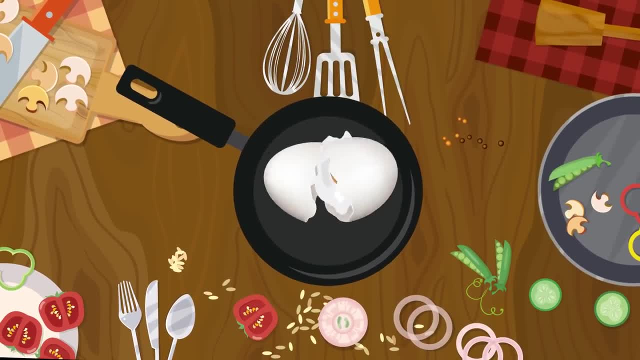 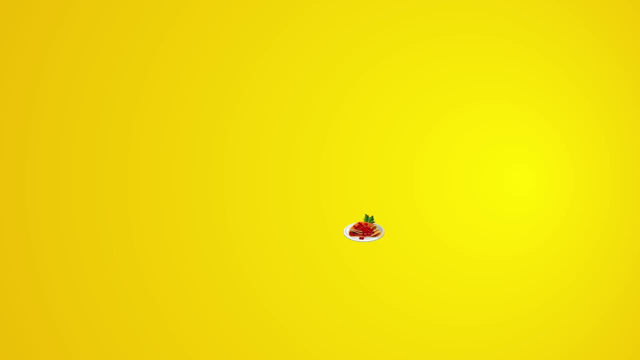 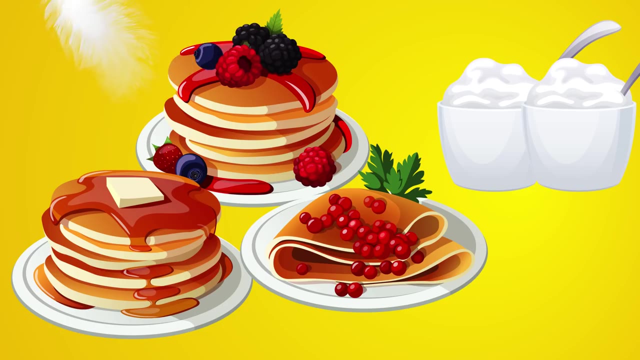 of the flavor Number seven, The best pancakes, Regardless of the recipe you follow, always add two tablespoons of sour cream to the mix. This trick suits all kinds of pancakes. Also, the best pancakes are likely to be type-A pancakes When you add the sour cream, a lot of sour cream, and then add the sweetened cream. 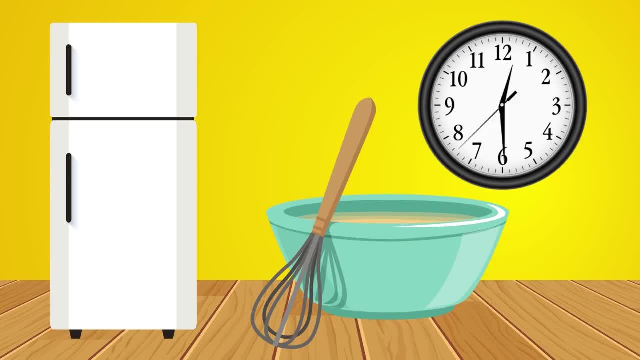 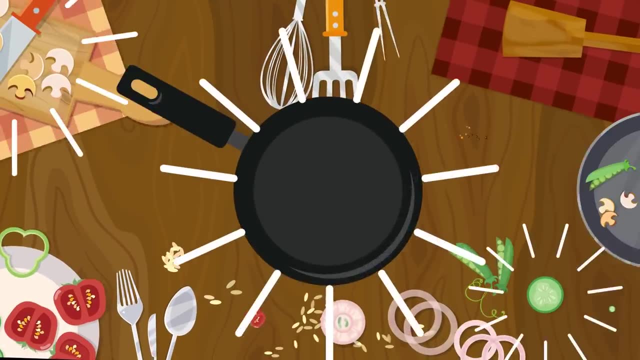 you end up with a very thick and velvety recipe, And these pancakes will make your pancakes taste so much better. The next tip depends on how good you think them are. The tastiest dough you can get is the one that has been kept in the fridge for about. 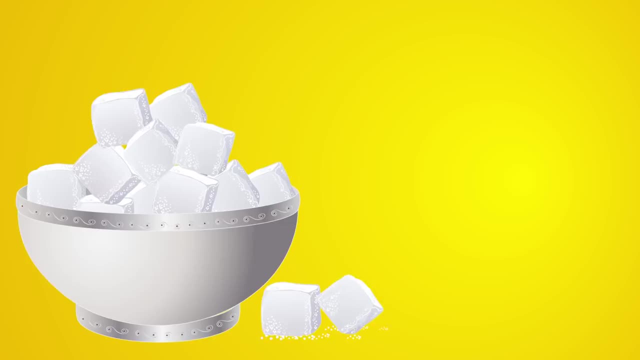 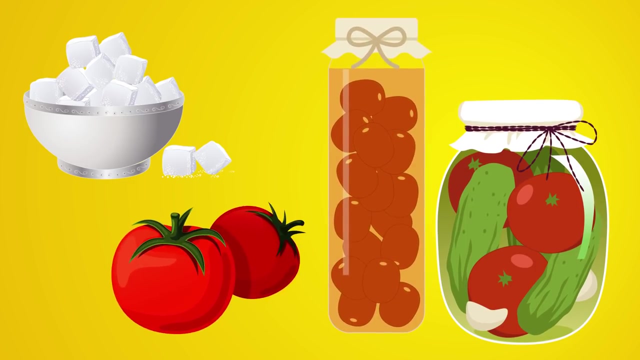 twelve hours. Are you in doubt, Check it out. Number six: Sugar is not just for sweetness. The perfect way to balance the sweet and salty taste of pancakes is to add sugar tomatoes or a tomato paste. The sugar reduces their natural sourness and makes any meal taste. 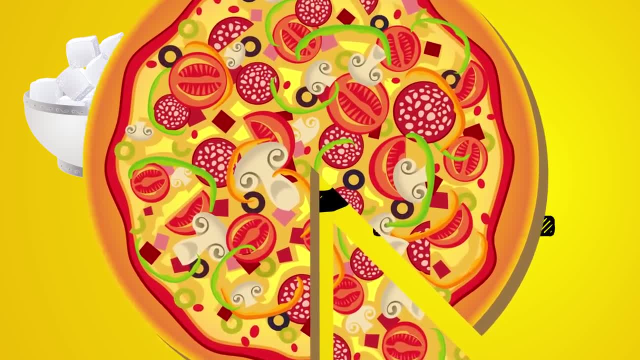 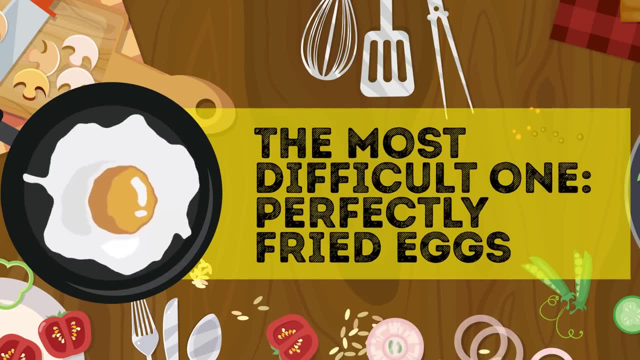 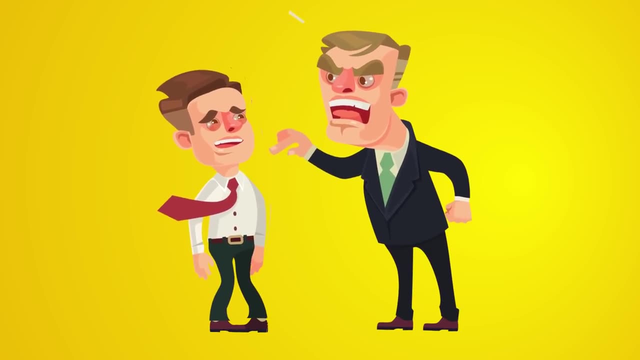 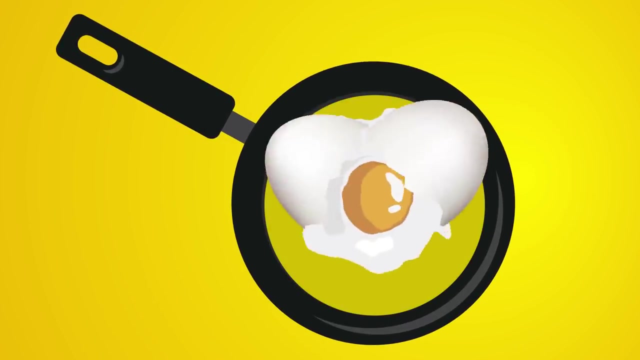 better, Just don't overdo it. Nobody wants a sweet pizza. Number five, the most difficult one: perfectly fried eggs. Anyone can fry an egg, you might say. Let us disagree. The three components of a perfectly fried egg are a thick-walled frying pan, butter and minimum heat. Heat up the frying. 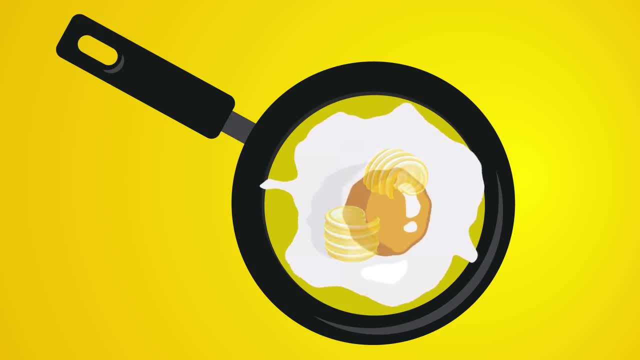 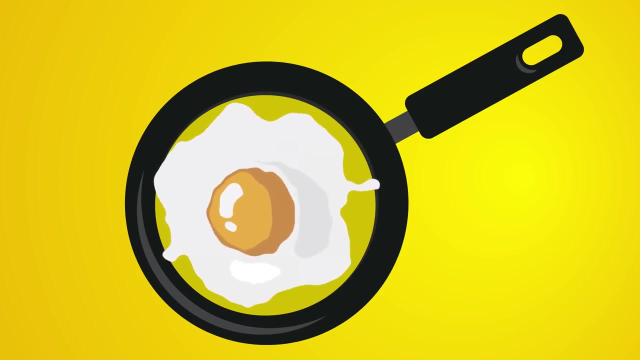 pan and add a half tablespoon of butter. It has to melt slowly, not reach a sizzle. Break the eggs and cook for four to five minutes. Add salt and enjoy perfectly fried eggs. Another variant is to melt some butter, then break an egg on top of it When you see that the bottom of the egg is already. 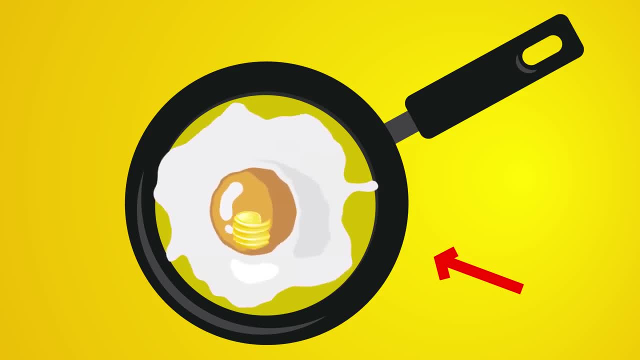 firm. the egg can slide around easily. add another piece of butter As soon as it melts. scoop a bit with a spoon and pour over the whites. Repeat this until no liquid butter is left. then sprinkle the egg with some salt. Bon appétit. 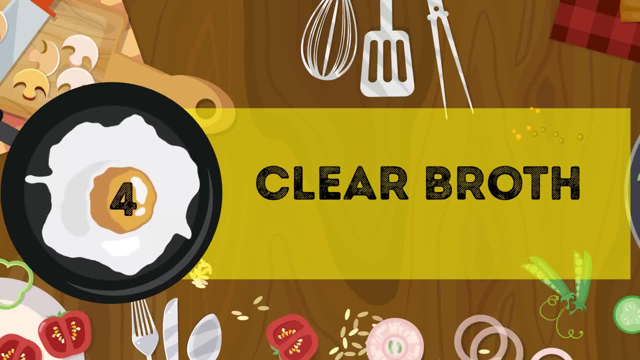 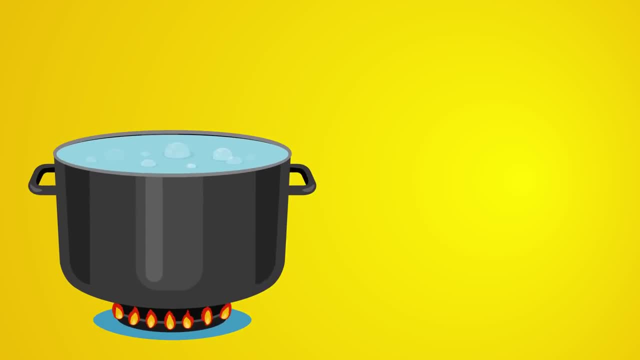 Number four: clear broth. A clear broth is the main component in many soups, sauces and other dishes. To make a crystal clear broth, you need to cook chicken on a low heat with a little bit of butter. If you don't have a 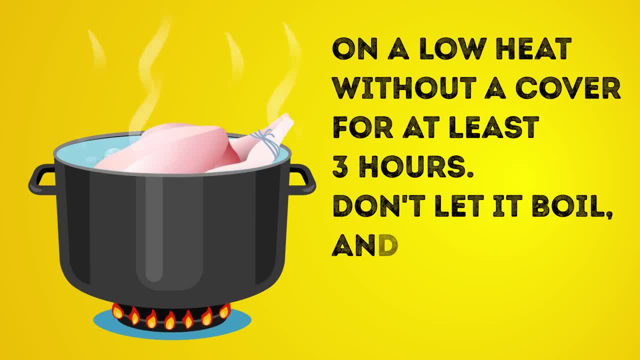 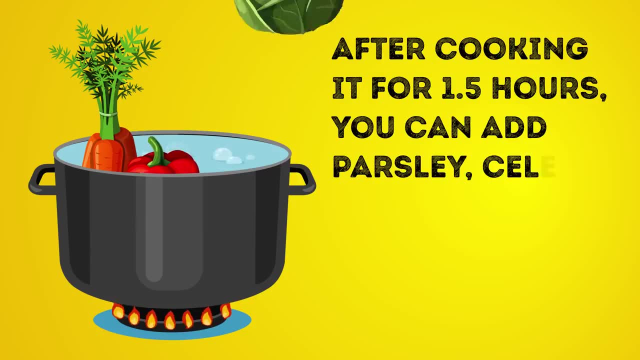 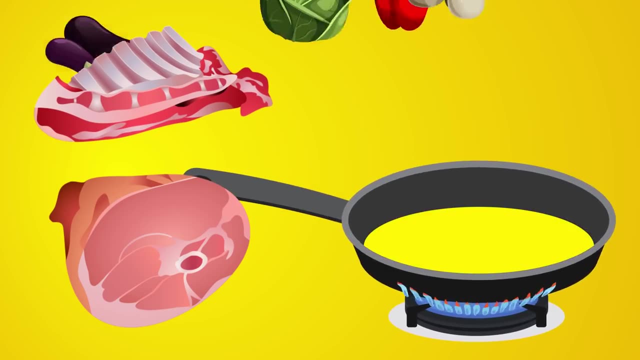 high heat. you can cook chicken without a cover for at least three hours. Don't let it boil and remove the suds as they appear. After cooking it for one and a half hours, you can add parsley, celery, carrots and onions. When cooking a beef or a lamb broth, you might want to roast root. 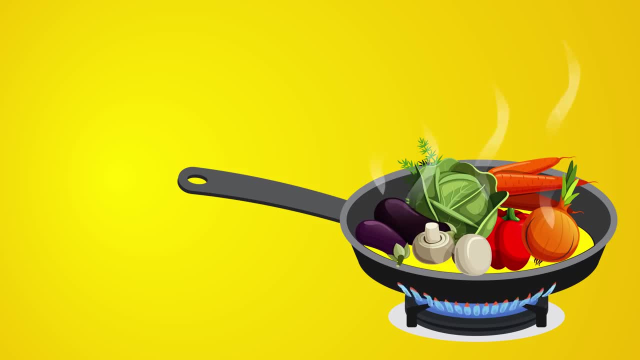 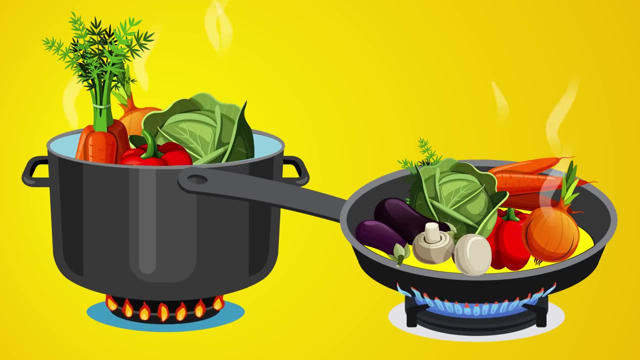 vegetables before adding them to your soup. Just cut them into halves and put them in a heated frying pan without oil. Fry until a dark brown crust appears and then add them to the broth. This trick will make the taste of your dish very rich. 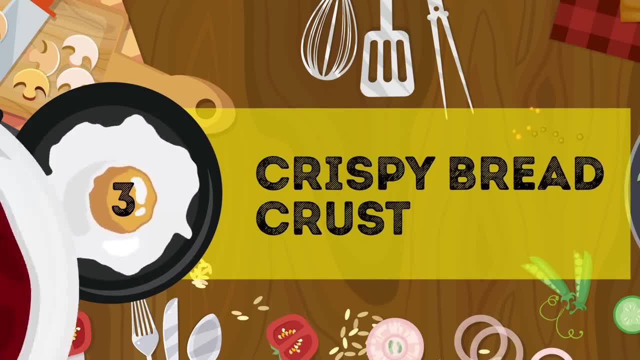 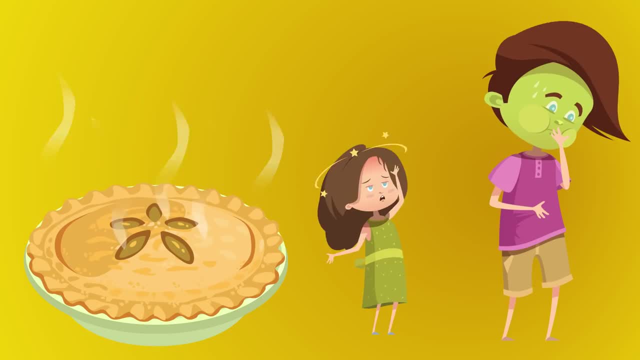 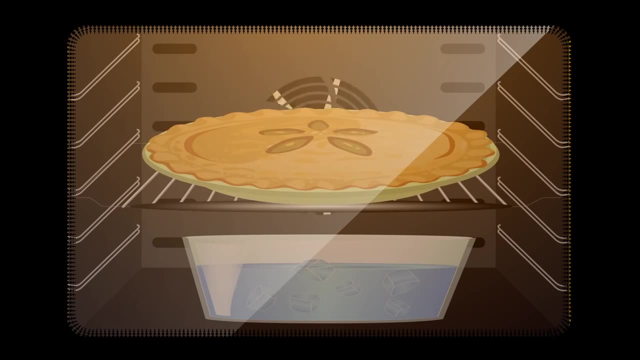 Number three: crispy bread crust. If you bake at home, you might have faced difficulties with your crust. It's either too pale or too thick. You can solve this problem quite easily by putting a bowl of water into your oven when you bake. Instead of such a bowl, you can use a tray full of ice cubes. 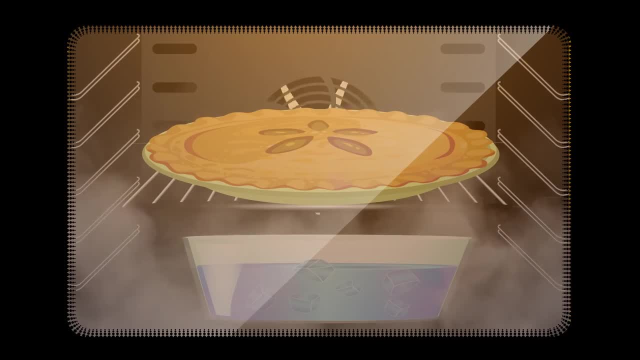 The trick here is in the same way. If you bake at home, you might have faced difficulties with your crust. Just open the lid and pour half of the water you have melted into your crust. This way, the crust will be cook too quickly and instead of being crispy, it will become burnt and 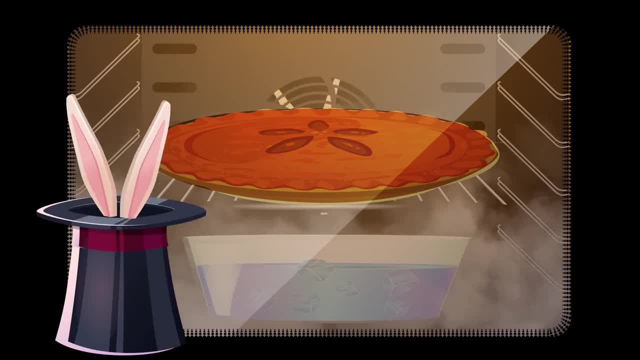 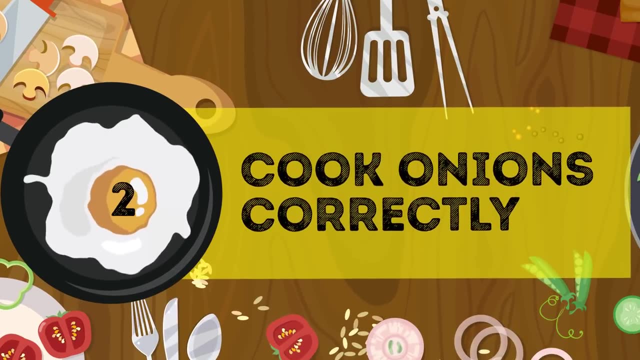 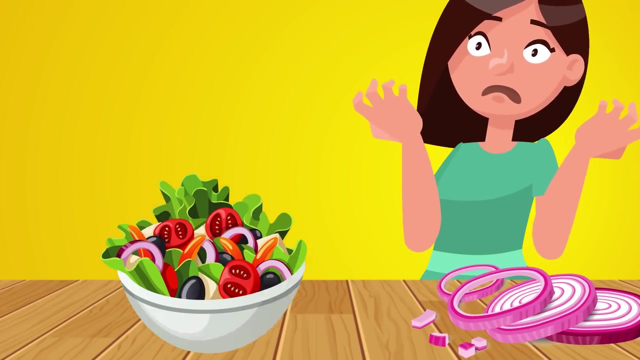 dense, The steam will do the magic and you'll have nothing to do but enjoy the results. Number two: cook onions correctly. Do you avoid using onions in your dishes because they turn out strange every time? If you have a little bit of a problem with your cooking, you can use this. 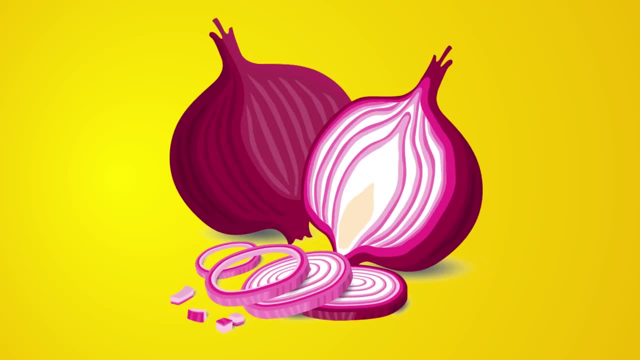 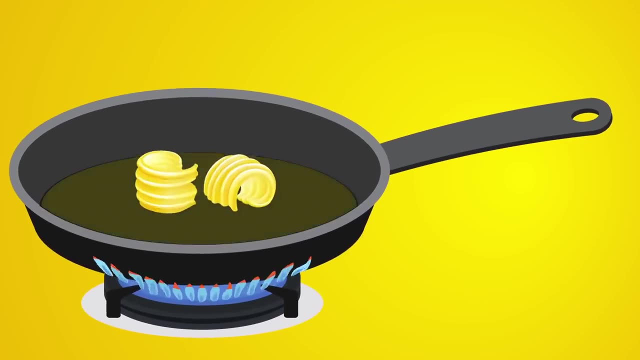 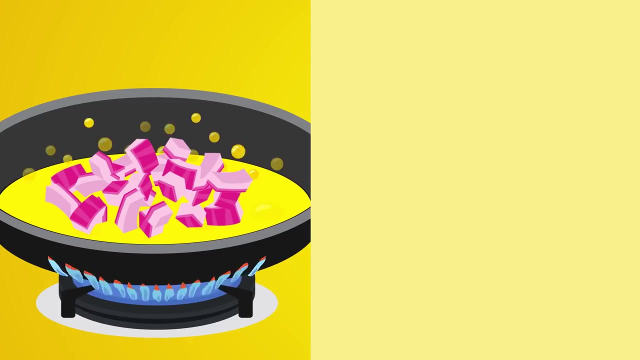 every time you try to cook them. forget this problem. we will reveal the secret of perfectly made onions for you. using a medium heat for frying and add both cooking oil and butter to the heated frying pan. cut the onions and fry them with some salt. the salt does three good things. it gets rid of the unpleasant 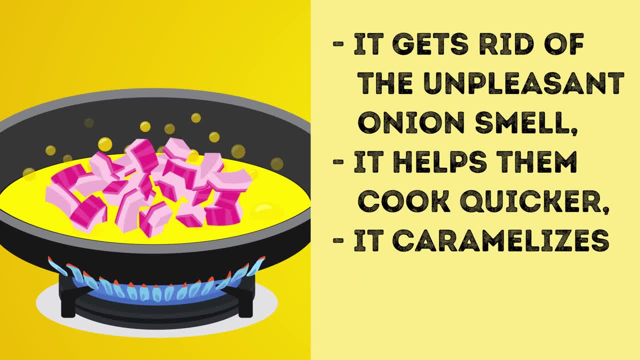 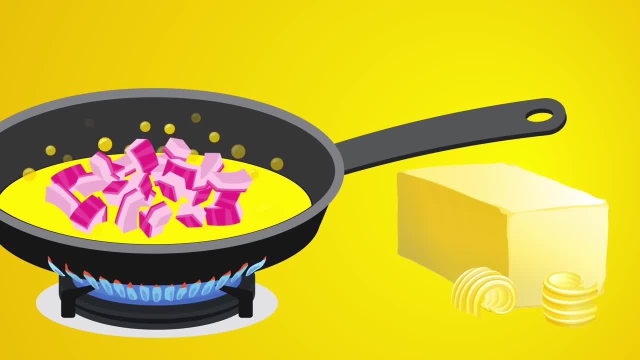 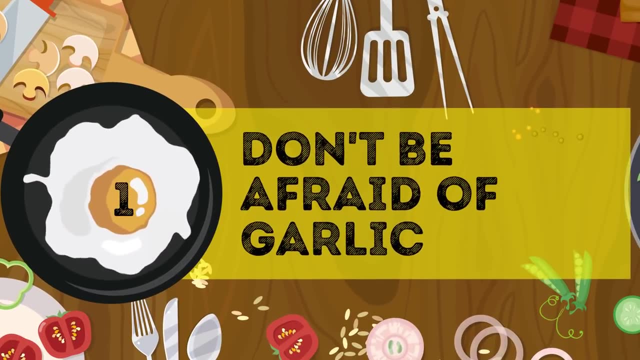 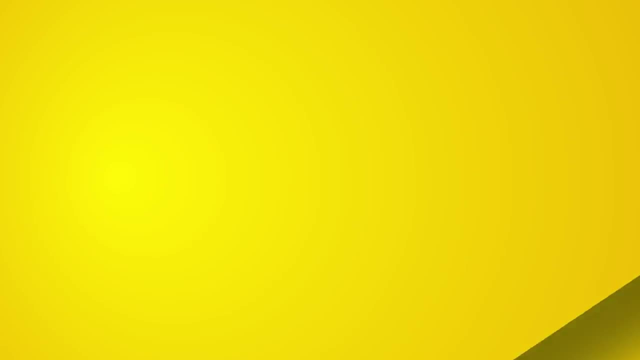 onion smell. it helps them cook quicker and it caramelizes them to add a sweet flavor. you should also only use butter for frying onions to prevent them from darkening. use melted butter instead. number one: don't be afraid of garlic. not only vampires are afraid of garlic. its smell can ruin a business meeting or a. 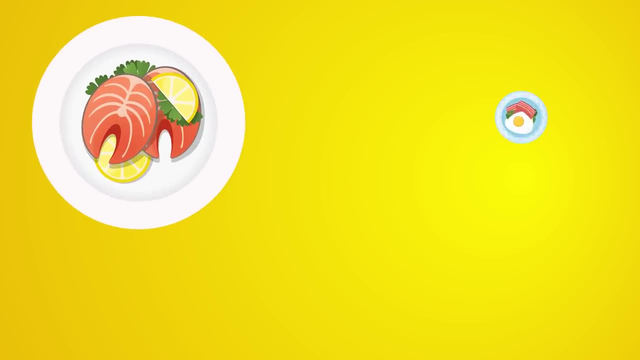 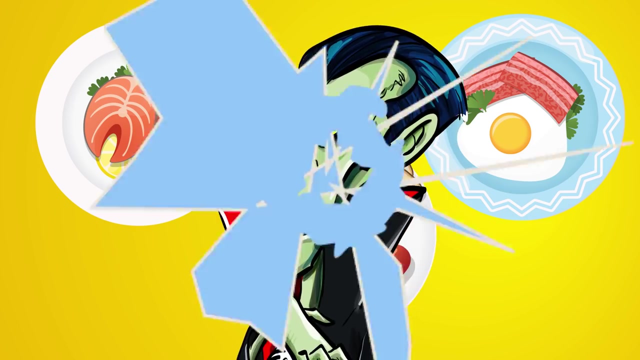 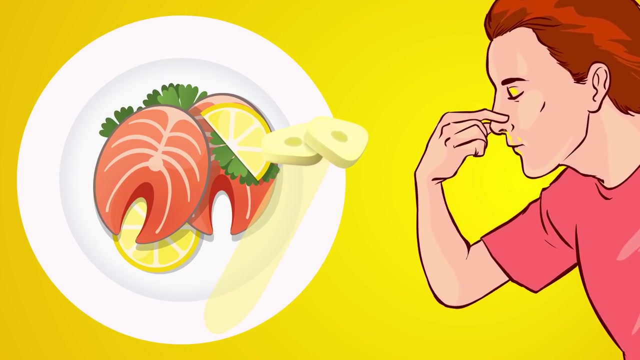 romantic dinner. if you still love to eat it but don't want to frighten away your date or wreck the negotiations- because who wants a partner terrifying vampires? don't add garlic to the dish. instead, you can apply some garlic juice to the plate. thus you'll avoid the unpleasant smell and enjoy your favorite. 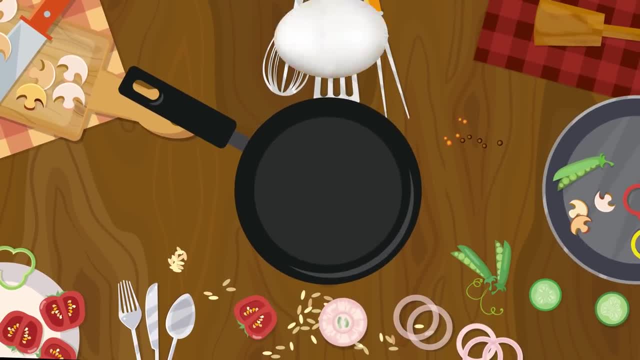 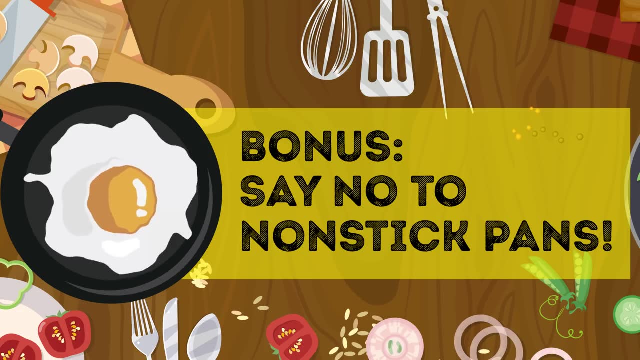 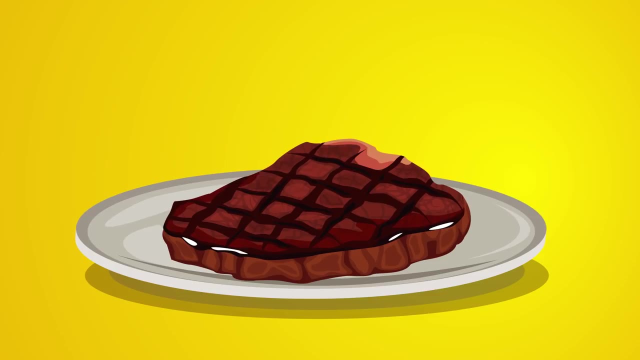 flavor. you are welcome. hopefully these tips have been useful for you. but there is one more secret left to reveal. bonus: say no to non-stick pans. have you ever noticed that it's quite hard to cook something with a crispy crust on a nonstick frying pan? the reason is the nonstick.